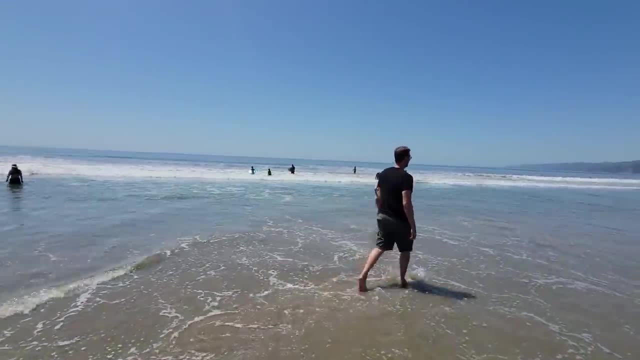 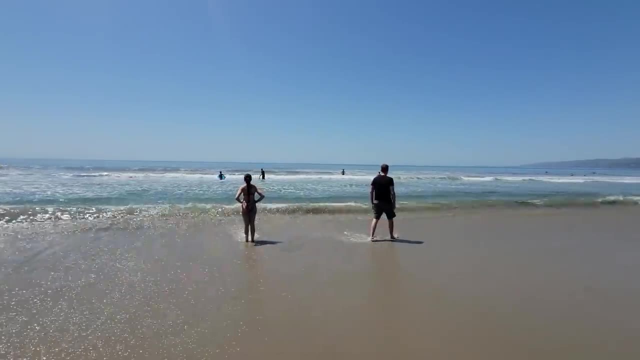 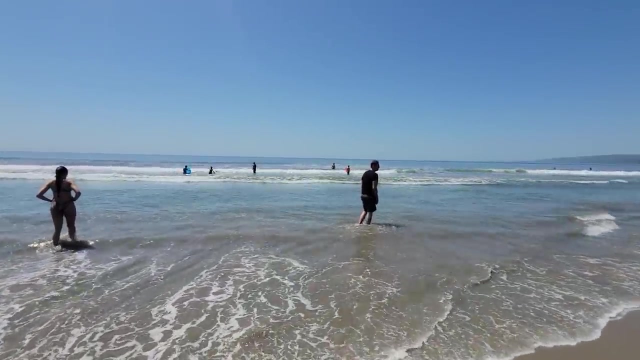 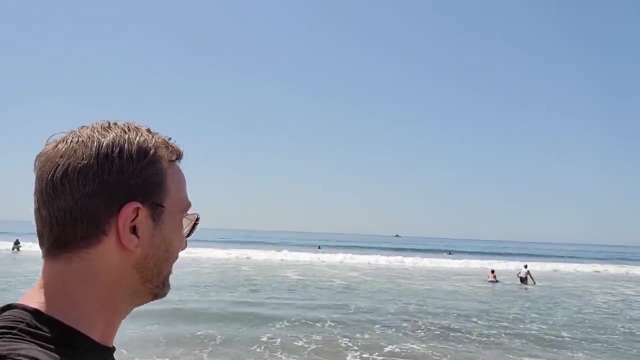 various hypotheses pertaining to humanity's origins are discussed at the university level. The out of Africa theory is heavily favored, despite compounding evidence to the contrary, because it seems to support a social engineering political agenda rather than a scientific one. Another theory which is touched upon is called the aquatic ape, which I covered in a prior video. 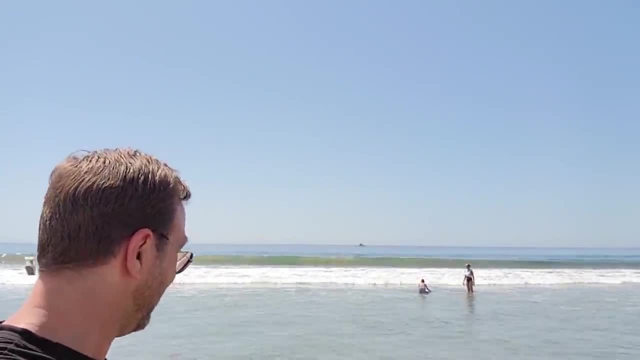 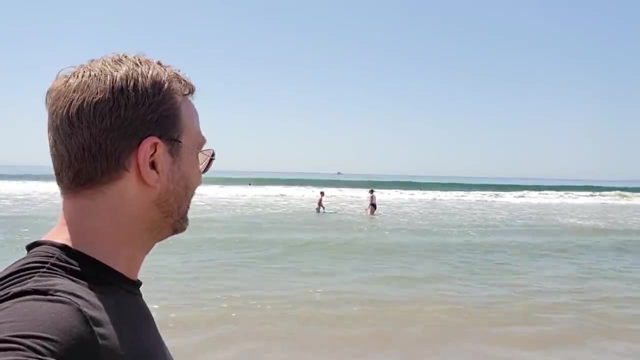 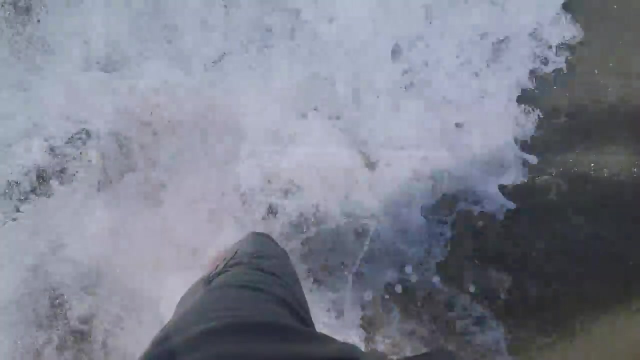 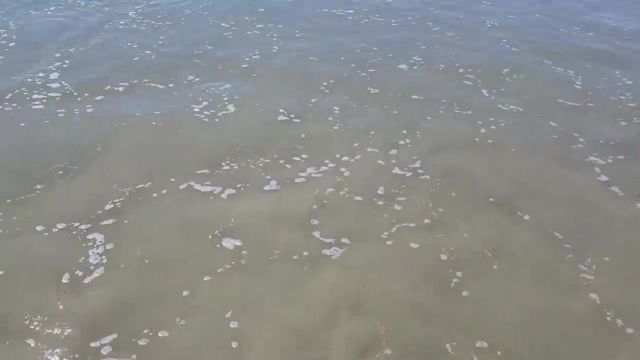 that postulates that mankind did not necessarily come about as a human being, but as a human being. A human being was a species of living creature that was found by the ancient alien being called Ithaca, and it's a genus of the sphagnum. 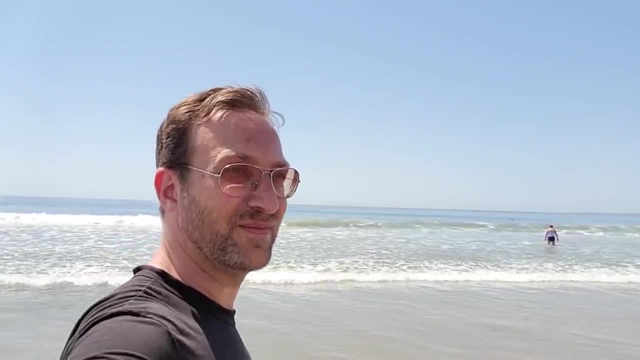 Many historians advocate that the Ithaca species as a human being may have not necessarily come about from monkeys and great apes, but may have shared a common ancestor that evolved around water, whether on the surface of the earth by lakes, rivers and oceans, or in subterranean caverns, which also contain similar bodies of water, with some upright walking hominins later taken to the trees to evolve into branch climbing monkeys or fur covered apes. And, while this may sound counterintuitive, I momentum this in a way that could be almost entirely hopeful if we take a closer look at the theory on this subject, something that has gone through the simmering of the entire process of January 2016, was certainly a betraying experience for the human species, both inside and outside of the university, as of December 2020.. 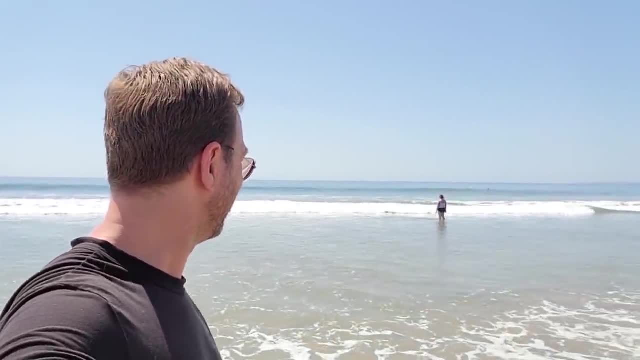 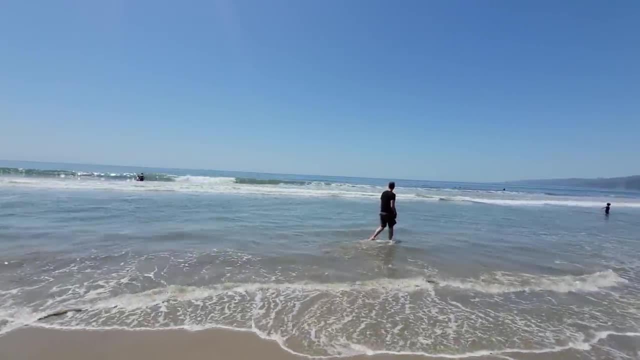 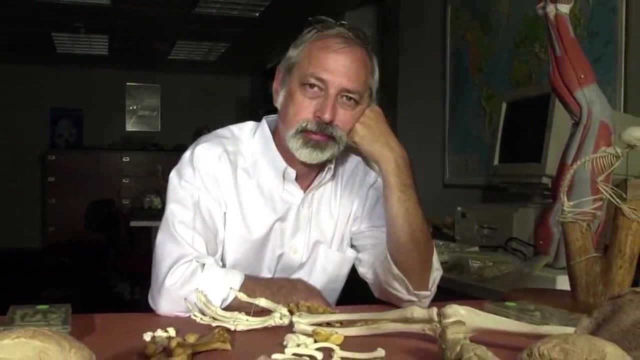 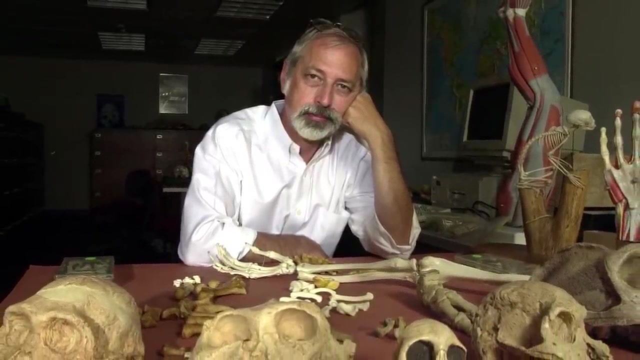 mainly because of decades of media conditioning. the concept does share some parallels among some of the world's foremost geneticists and evolutionary biologists, who may or may not also have received a coupon at red lobster. dr owen lovejoy is a distinguished evolutionary anthropologist at kent state university, ohio, best known for his work on australopithecine. 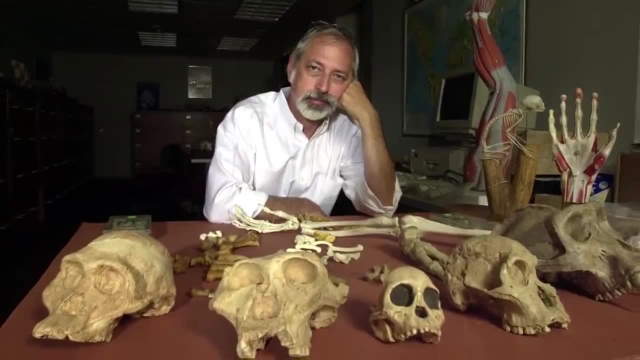 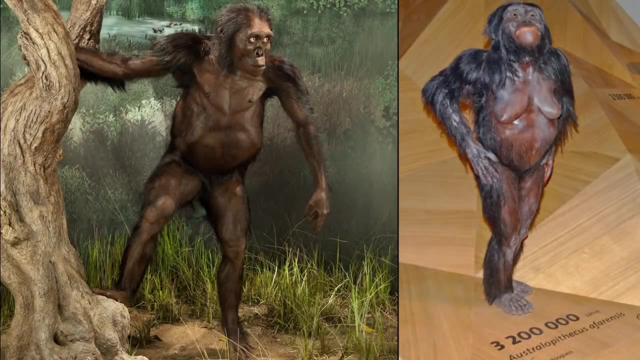 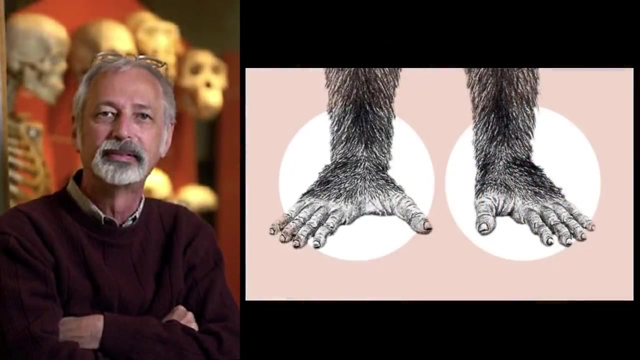 locomotion and the origins of bipedalism. lovejoy has published more than a hundred articles related to his research and is most well known for his work on reconstructing lucy, an alleged human ancestor with an opposable big toe on its feet, meaning they resembled thumbs for grasping. 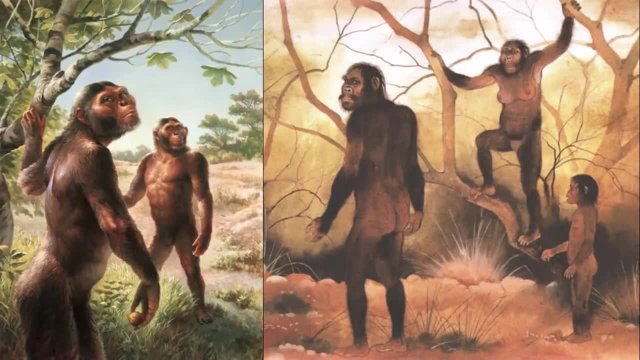 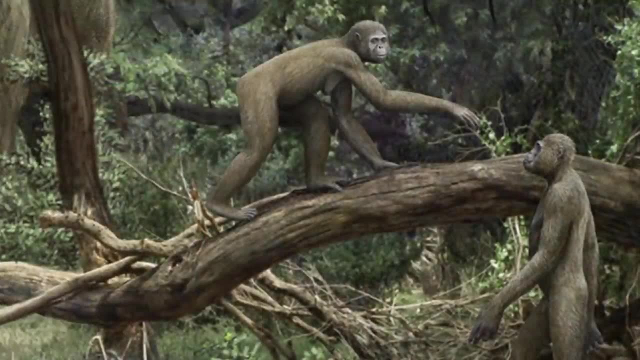 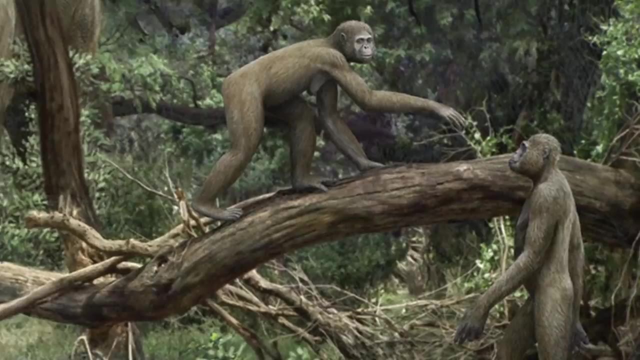 branches and climbing trees. while lovejoy claimed that lucy, which was dated to 3.4 million years ago, was at least partially bipedal, he proposes that artie, another alleged human ancestor dated to between four and five million years ago, spent more of its time allegedly walking than lucy, despite being over a million. 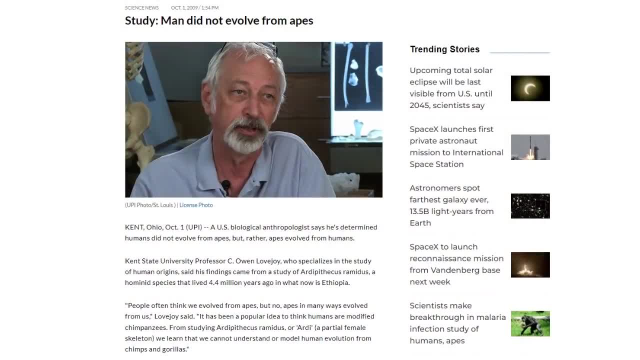 years older. this article, titled man did not evolve from apes, says a us biological anthropologist, says he's determined: humans did not evolve from apes, but rather apes evolved from humans. you, Kent State University professor C Owen Lovejoy, who specializes in the study of human origins. 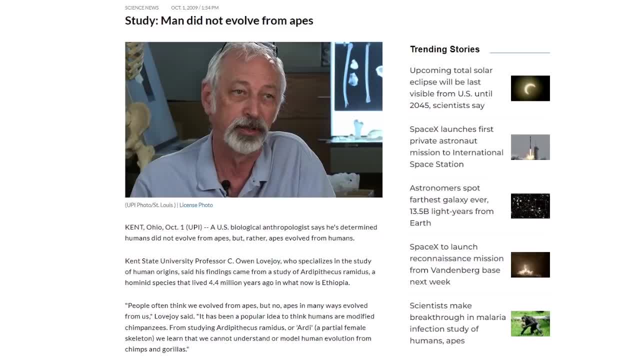 said his findings came from a study of Ardipithecus ramidus, a hominid species that lived 4.4 million years ago in what is now Ethiopia. Quote: people often think we evolved from apes, but no apes in many ways evolved from us. Lovejoy said It has been a popular idea to 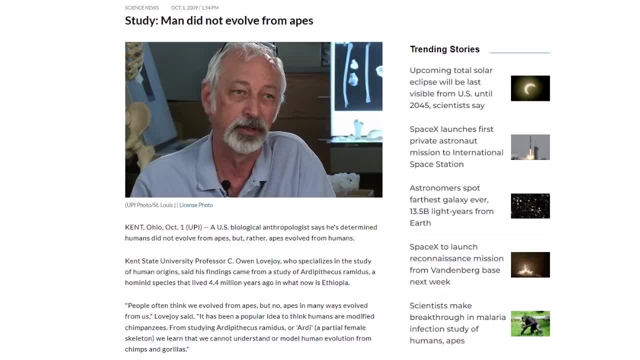 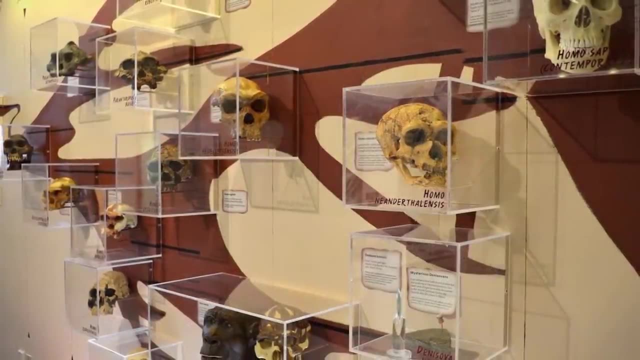 think humans are modified chimpanzees. From studying Ardipithecus ramidus or Ardi, a partial female skeleton, we learned that we cannot understand or model human evolution from chimps or gorillas. Of course, Lovejoy is still very much in the mainstream, and while he proposes that 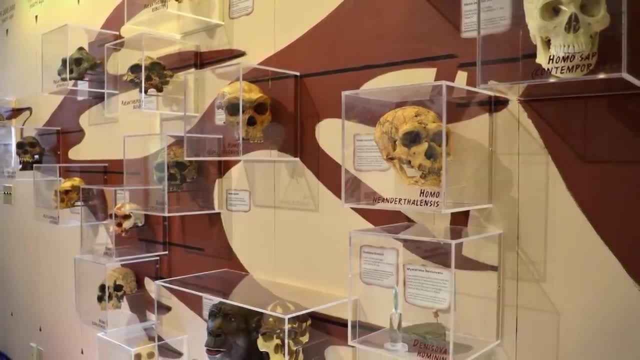 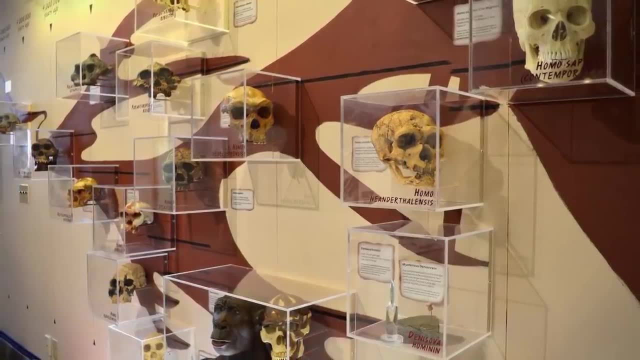 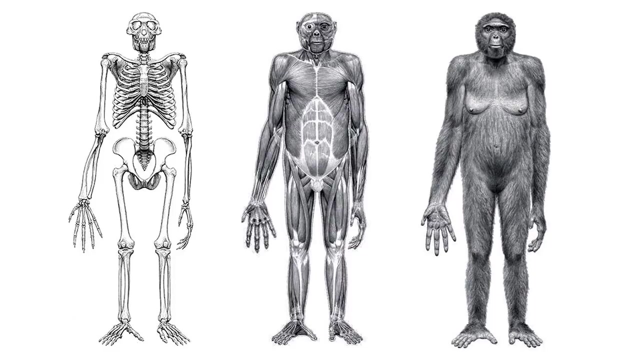 humans and apes shared a common ancestor that was neither human or monkey, at least he makes it. modified chimps is false. My own analysis is that neither Lucy or Ardi, which were a little over three feet tall, walked upright at all and were both primarily tree dwellers. not only because 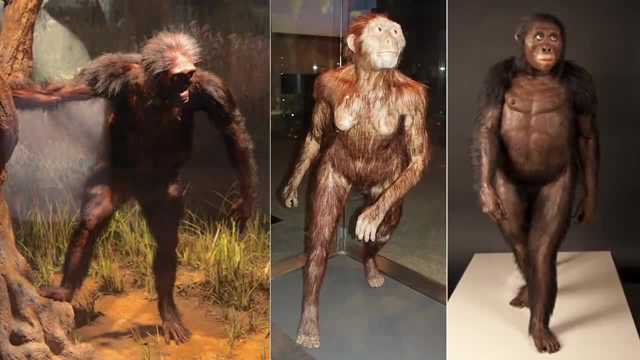 their feet resembled hands like other apes, but because their furry ape-like bodies did not sweat the way all bipedal hominins do, as sweating is a trait that is associated with running and hunting, which neither of these specimens did. The artistic reconstructions in museums are deceptive. 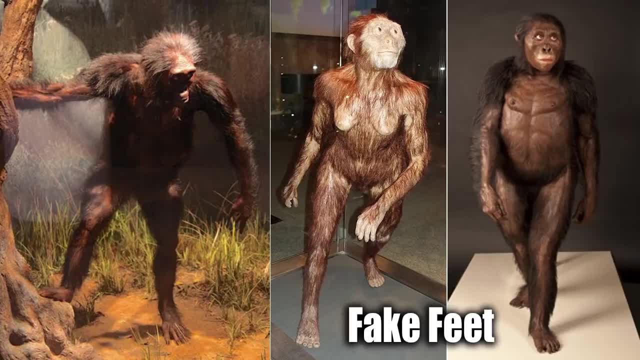 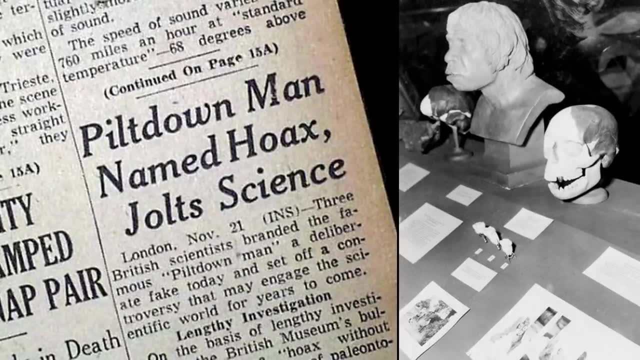 showing erect upright models with human-like feet, which is a fraud, and while they're not completely fake, specimen like the Piltdown Man, which was a baboon's jaw glued onto a human skull and touted as the missing link by the British Museum for almost 50 years, or the Nebraska Man, 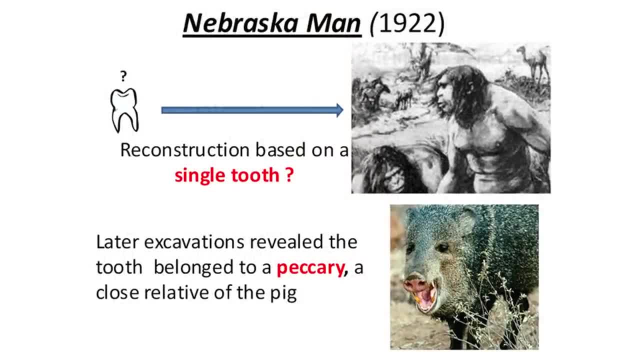 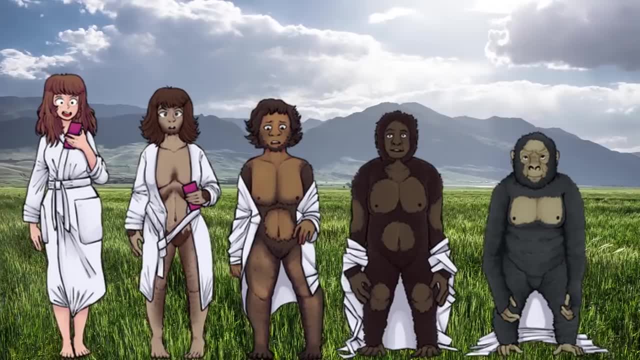 which was another imaginary creation in the 1970s. they were all based on what turned out to be a pig's tooth. The missing link is still very much missing and the linear hominin progression proposed by the out-of-Africa model. 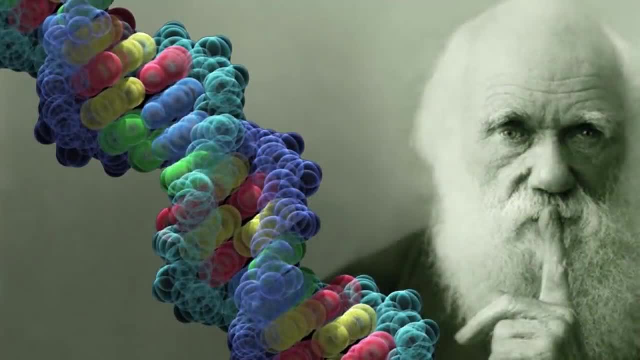 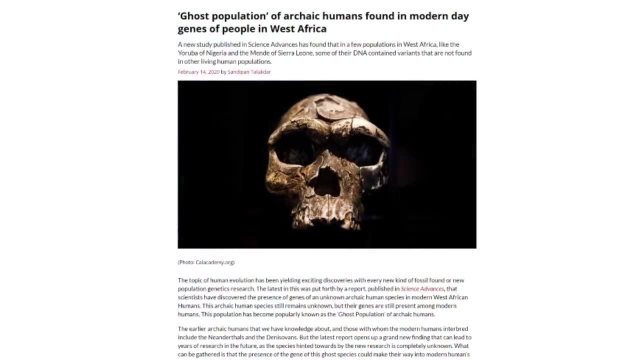 continues to fall apart as advances are made in the field of genetics. The obsolete and politically motivated out of africa model proposes a single and relatively recent transition from archaic hominins to anatomically modern humans. I'm sure you're all familiar with this, but long agoチャンネル. I don't know if you know인데 who is involved in this, but I think he is Next to me- is Chris Cotillard, a famous geek who was living in the mid-19th century but a member of the British Museum of. 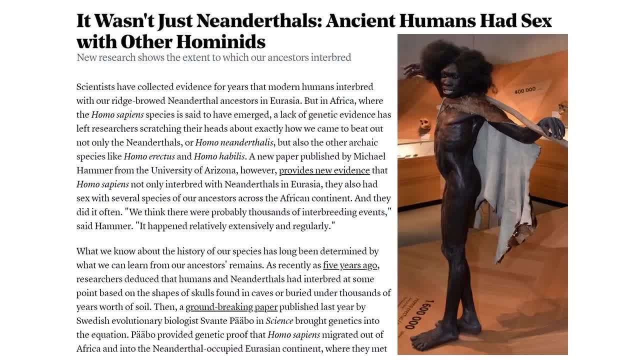 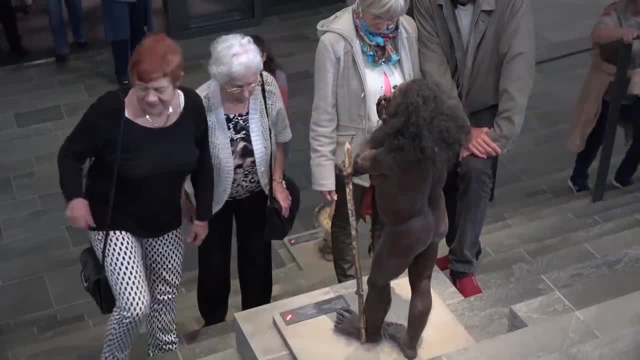 Geography, who had access to this jamaaa in the middle of the 90s, by the 18th century, until he was. humans in Africa, which is not supported by the fossil record, followed by a later migration to the rest of the world, replacing other still existing hominin populations, which again is 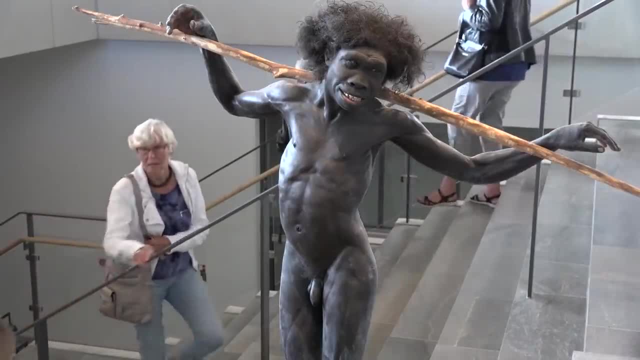 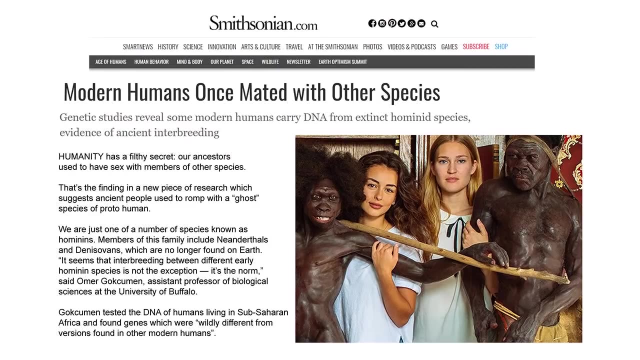 not what happened. DNA sequencing of modern and archaic genomes has now conclusively and irrefutably demonstrated that humanity is a hybrid species and that racial differentiation exists because we're comprised of various degrees of different hominin species which interbred within the past 50,000 years. In this article published in Nature, we read that ancient humans 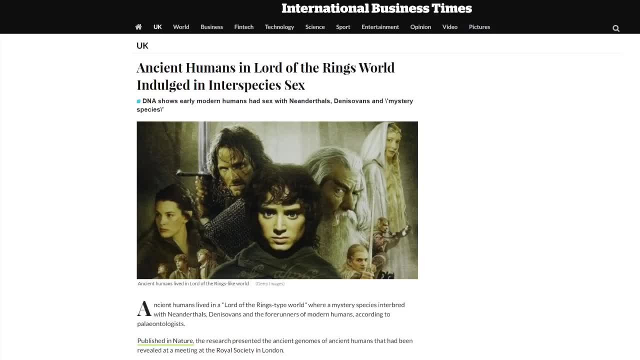 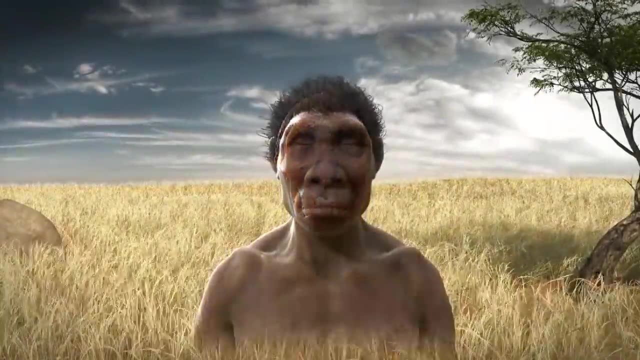 lived in a Lord of the Rings world and indulged in interspecies sex, including male and female, Neanderthals, Denisovans and a mystery species which anthropologists have labeled a ghost species, meaning it's considered super archaic, not yet identified in the fossil record. but 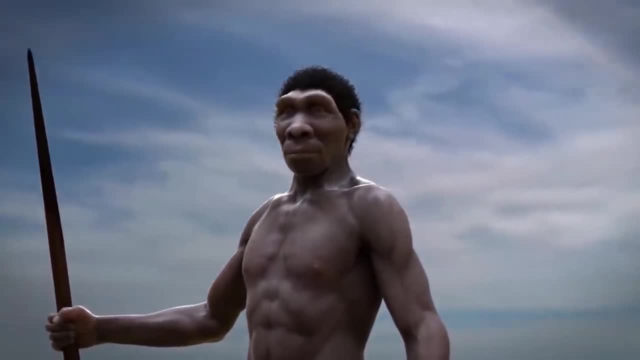 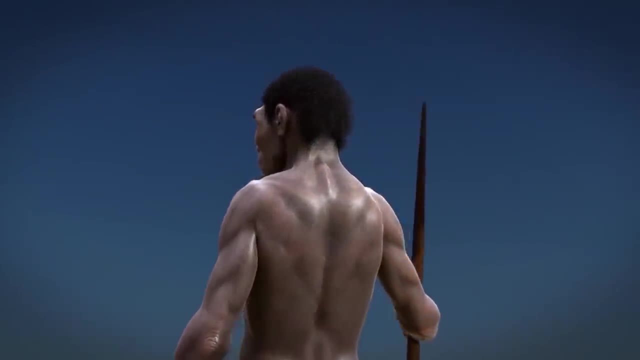 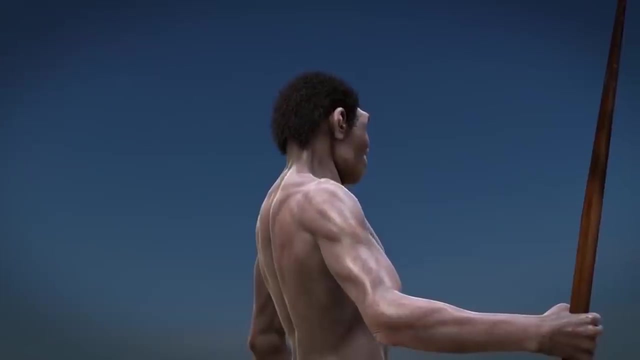 likely Homo erectus or Homo habilis, over 1 million years removed from modern hominins and comprises up to 19% of sub-Saharan African DNA not found in the DNA of Asians or Caucasians. This interbreeding event happened about 43,000 years ago in Africa. In other words, it's not 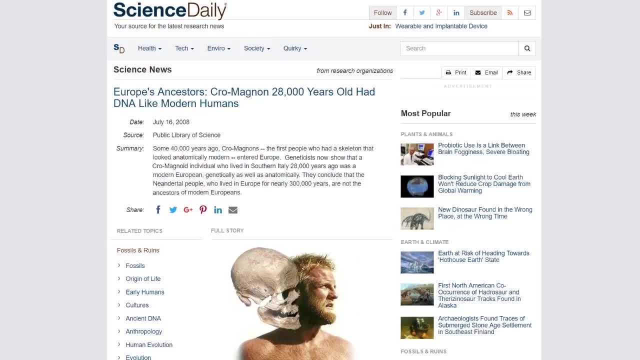 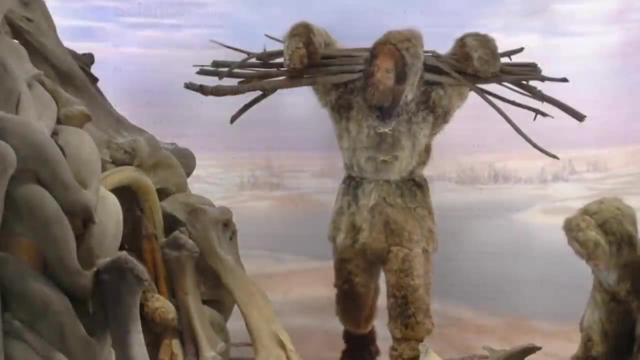 possible for sub-Saharan Africans that contain this archaic DNA that is absent in Cro-Magnon to have left Africa 35,000 years ago and magically mutated into what became modern-day Europeans, or Caucasians or Asians. So this leaves the question: where did Cro-Magnon or modern Europeans? 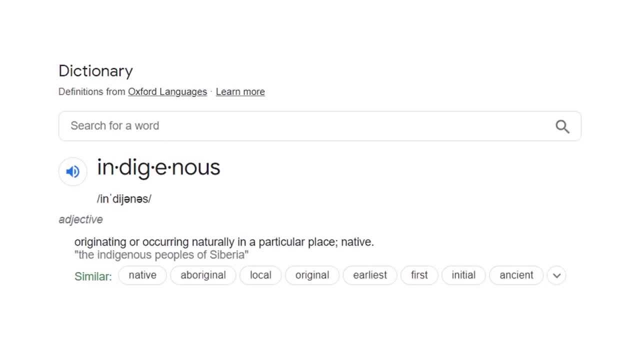 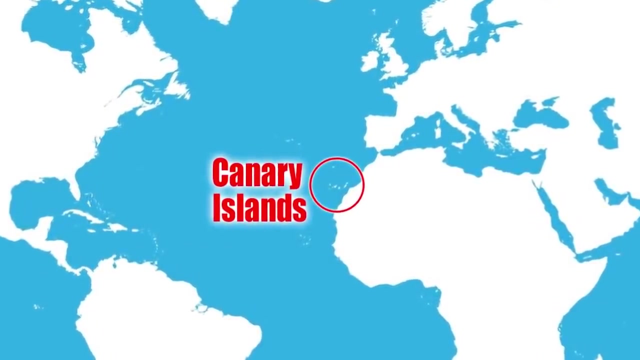 come from. When we look up the word indigenous in the dictionary, it says- quote: originating or occurring naturally in a particular place, native. That said, the islands right off of the coast of Africa are known as the Canary Islands, and the native indigenous inhabitants were known as. 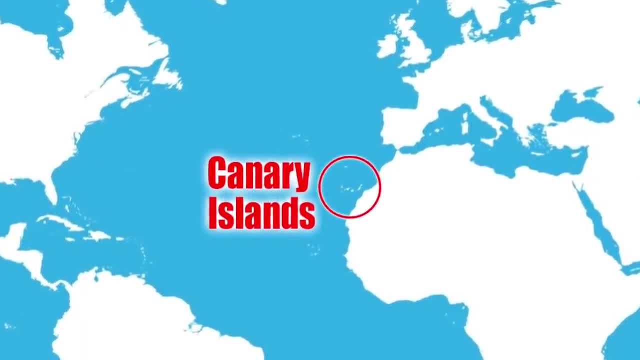 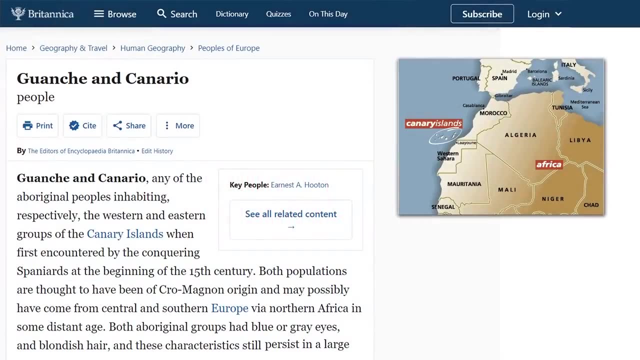 guanches. They left behind tall blonde and red-headed mummies and were studied extensively by the National Socialists of the 30s and 40s. If we look up the guanches in the Encyclopedia Britannica, it says that they were the direct 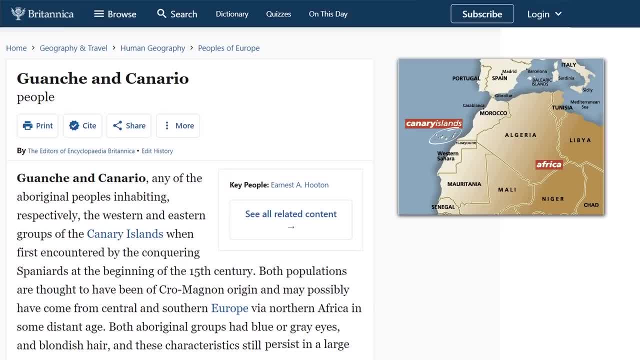 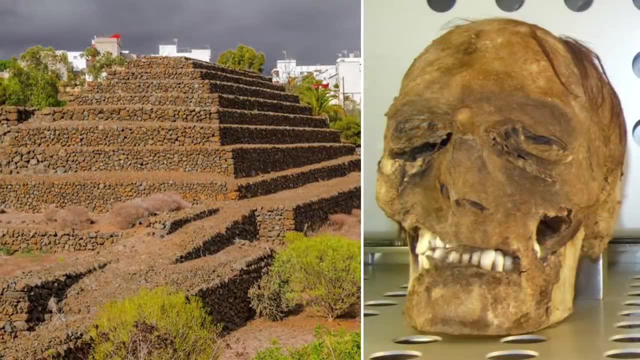 descendants of Cro-Magnon, which makes sense, as the museum on the Canary Islands has the largest collection of Cro-Magnon skulls anywhere in the world. It also says that they had blue or grey eyes and blonde hair, which also makes sense, since the mummies that they left behind. 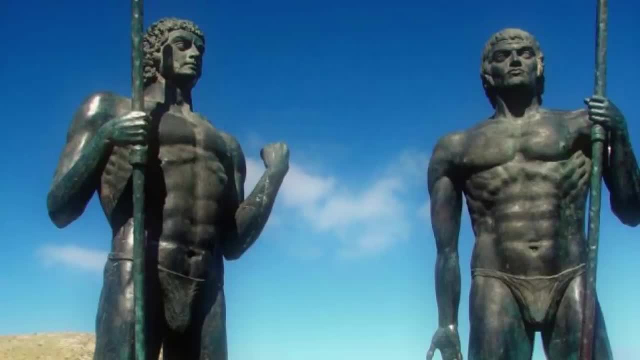 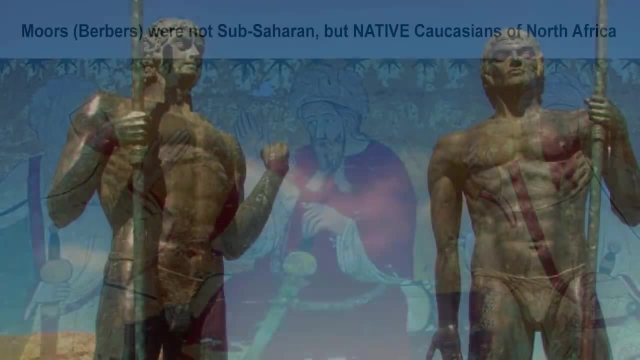 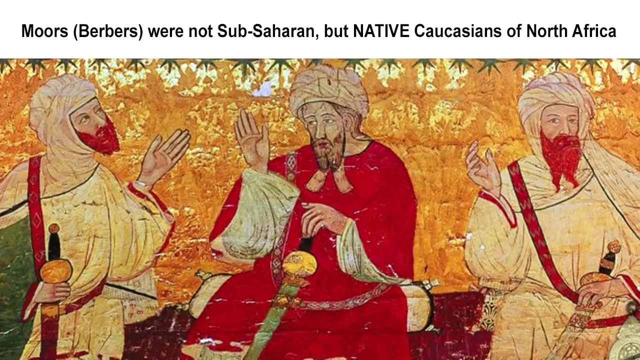 had blonde and red hair. It also links them to populations in Europe and North Africa, and not only do the guanches share genetic affinities with the Basque and the Berbers, which are the natives of North Africa, all of these populations are among the highest percentage of Rh-negative. 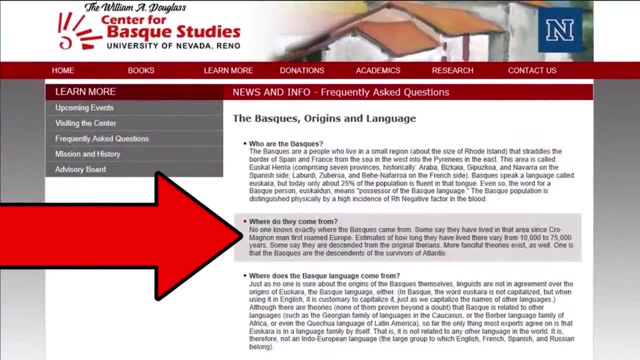 blood factor in the world. That said, the Basque mythology which, according to the Center for Basque Studies at the University of Nevada, says, quote: where did the Basque come from? No one knows exactly. Some say they have lived in that area since Cro-Magnon man first roamed Europe. Estimates: 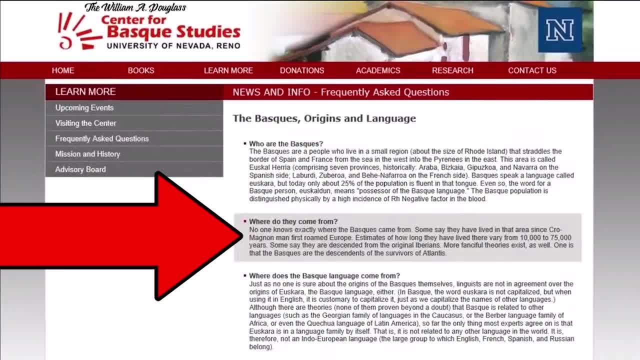 of how long they have lived there vary from 10,000 to 75,000 years. Some say they were descended from the original Iberians. More fanciful theories exist as well. One is that the Basque are the descendants of the survivors of Atlantis. 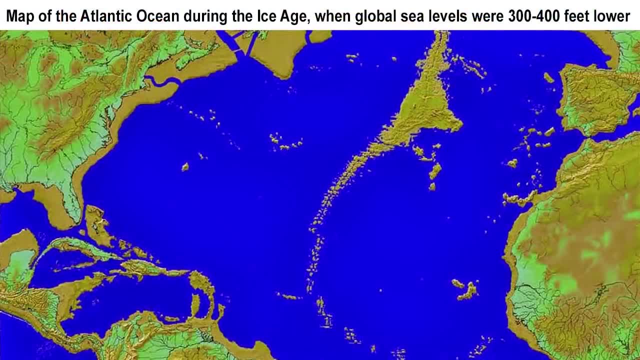 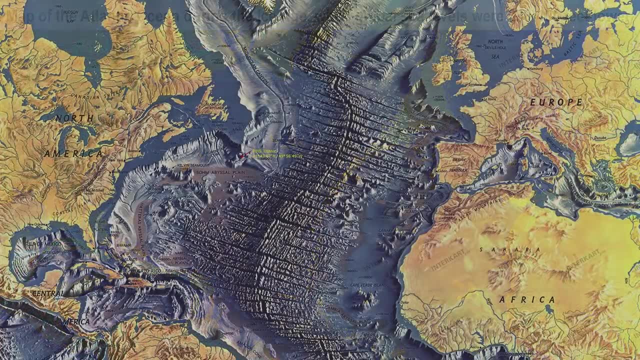 The concept of Atlantis becomes less fanciful and more probable when one looks at plot points and at apocalyptic maps. These are maps of the Ploistocene, or ice age, maps of the Atlantic Ocean, when Atlantis was said to have existed and sea levels were much lower or genetic. 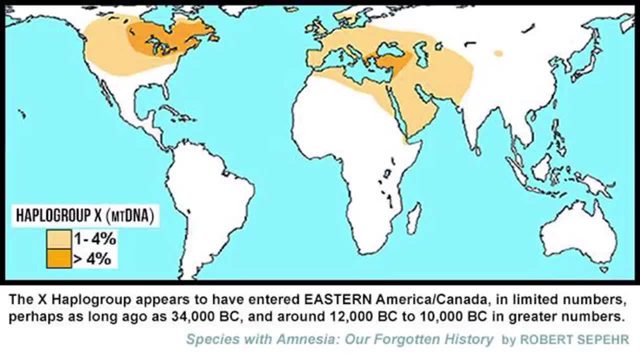 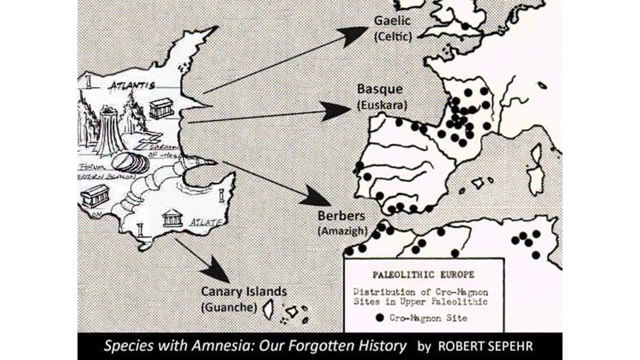 maps of the Ploistocene distribution of DNA on both sides of the Atlantic, such as Haplogroup X, But we never hear about these perspectives because the people that controlled the media and academia in the 21st century are the same people that were promoting the Piltdown man. hoax during the 20th century. What, in fact, are the people? Or are these people the people that were capable of doing things, Or are these people the people that were capable of doing things? Or are these people the people that were capable of doing things, Or are these people the people that were? 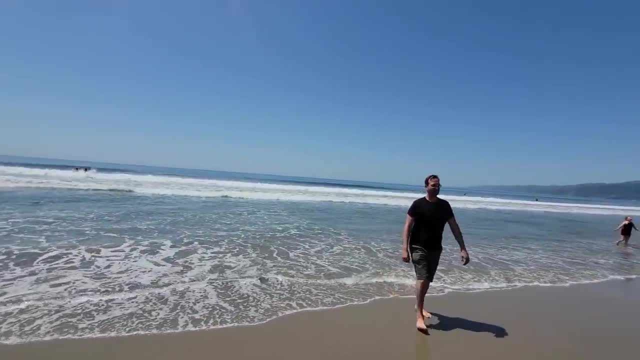 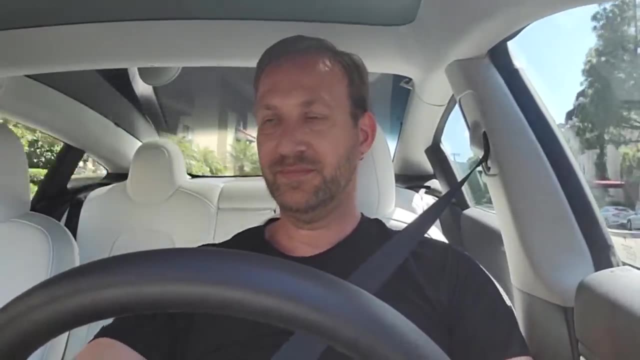 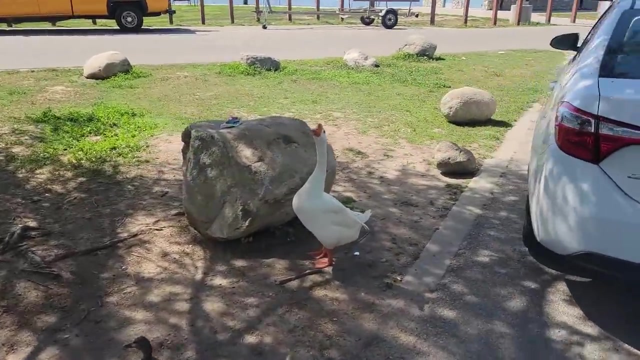 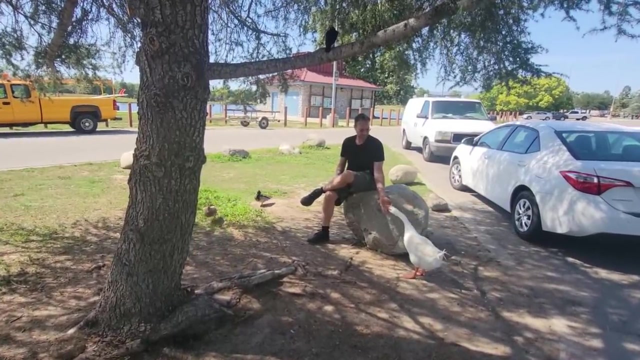 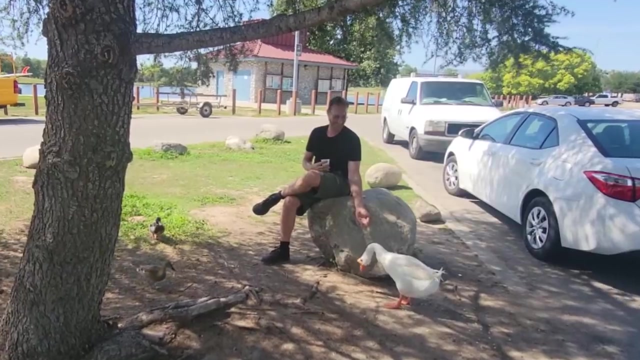 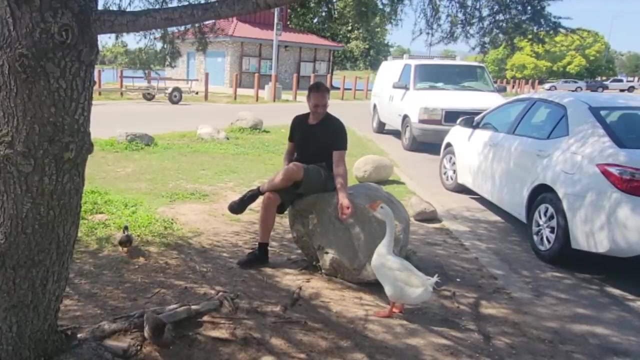 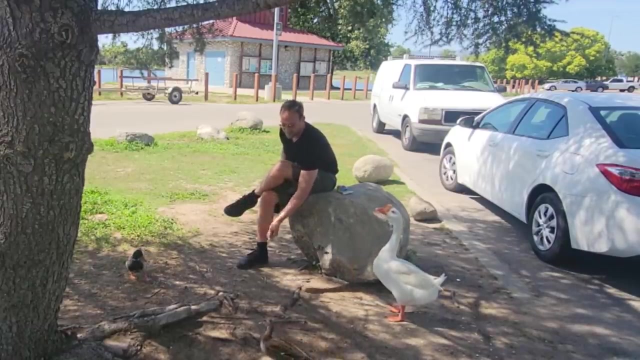 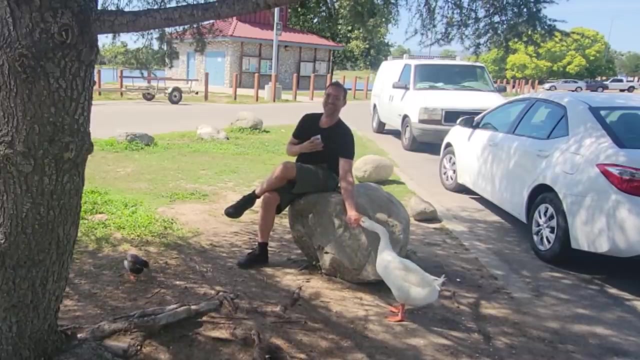 century. I have a lot more to say on the subject, but I'm starting to get hungry and also wanted to visit my favorite goose before I cash in my coupon, who I think is finally starting to warm up to me. I've been coming to this park for several years now. 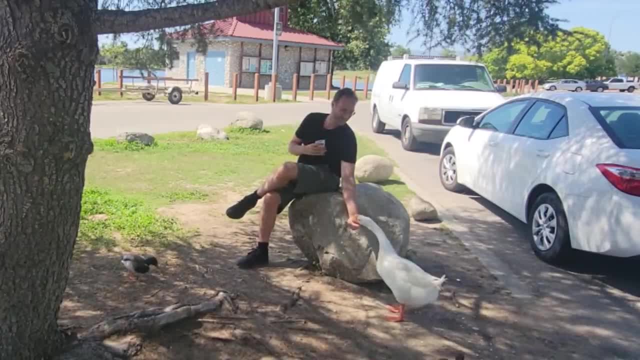 and this is the first time I've been here. It's a great place to get some fresh air. This is the first time I've been here. It's a great place to get some fresh air. first time that this goose has eaten anything that i gave him, let alone right from my hand. it just 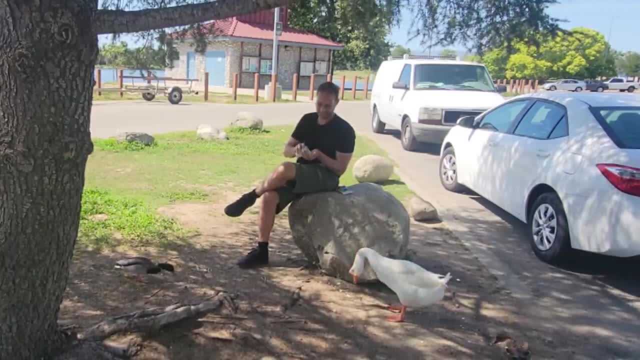 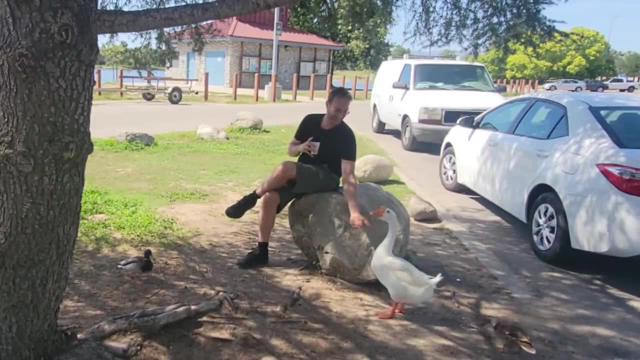 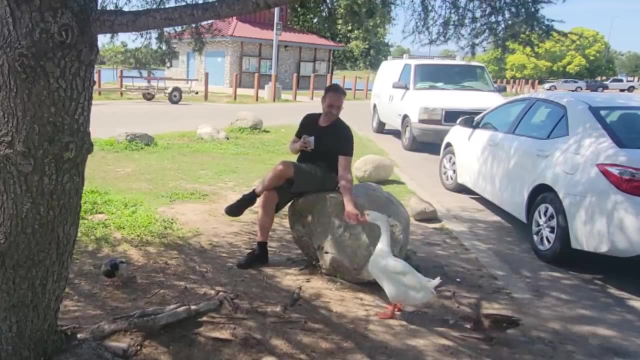 goes to show that, just like other things in life, most things can be accomplished with perseverance, and that includes the field of anthropology, which currently is in a dark age of ignorance and political dishonesty, but i'm confident that this too will one day change and humanity will. 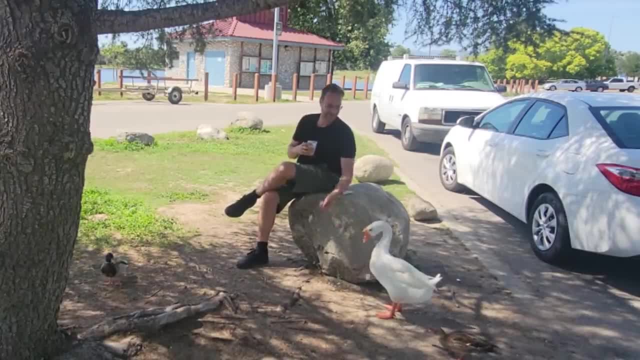 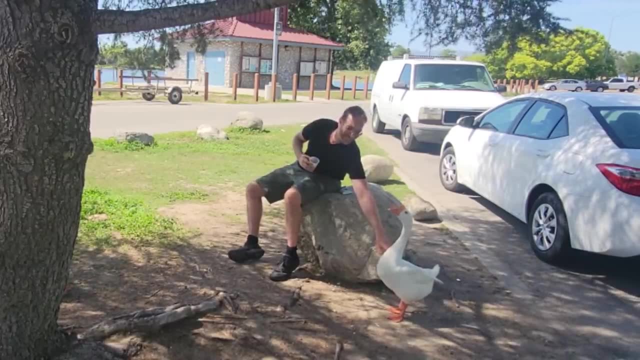 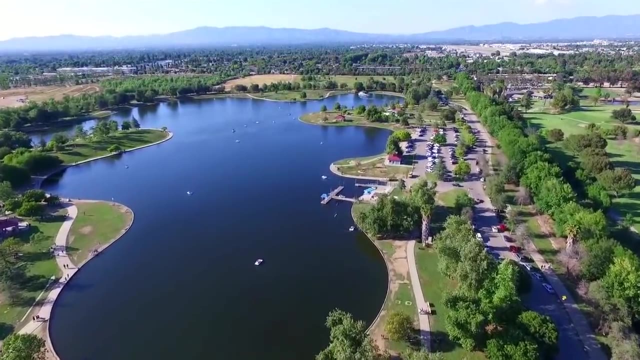 discover that not only is its history much more interesting than we're led to believe, but there's much more to mankind than being an alleged hairless ape. there's a much higher spiritual potential which we've forgotten but hopefully will soon awaken from our collective amnesia. 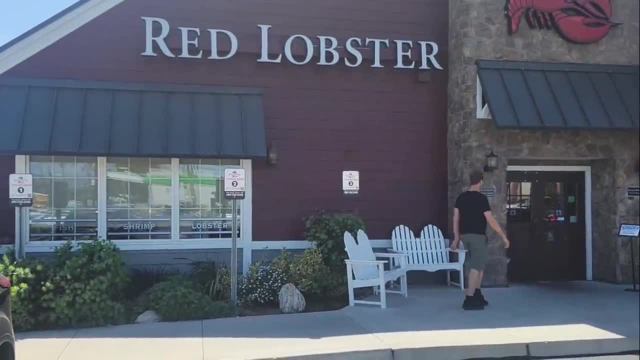 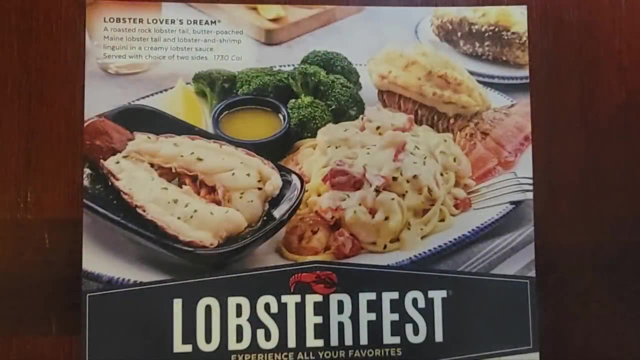 now that i fed the birds, it's finally time to give this place a try. it's my first time and i have high expectations. my waiter suggested that i tried the lobster lovers dream, which looks like it's high in cholesterol, but i decided to make an exception.